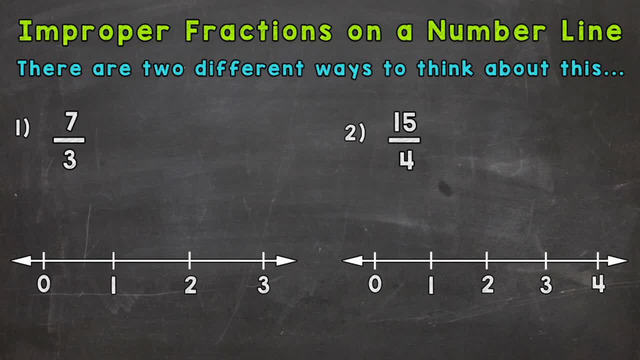 And the first thing that we should do is convert to a mixed number. So how many whole groups of three can we pull out of seven? So we can pull two whole groups with one left over. keep our denominator the same, So two and one third. 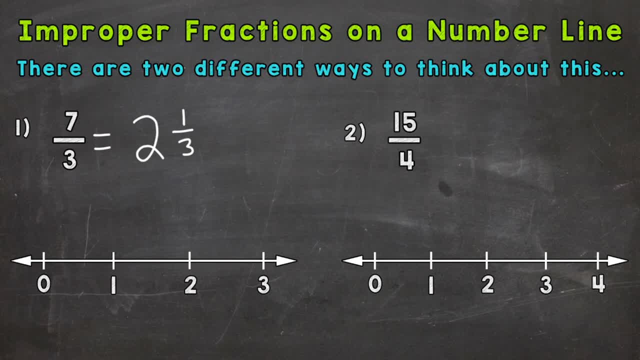 If you need help with converting improper fractions to mixed numbers, I have a video on that. I dropped the link down in the description, So now that we have the equivalent mixed number, it's going to be easier to place that on a number line. 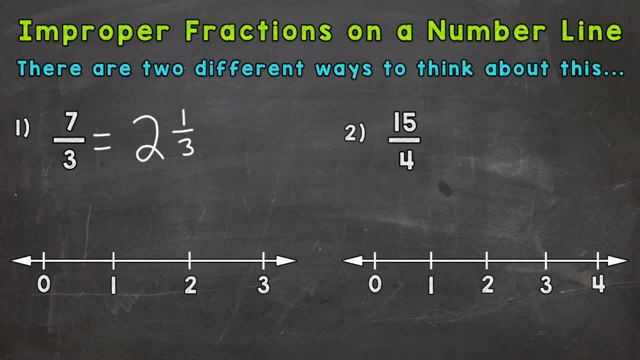 So we know two and one third is going to be between two holes and three holes, So this portion of the number line, So we need to split that into thirds or three equal sections because of our denominator We have two plus that one third. 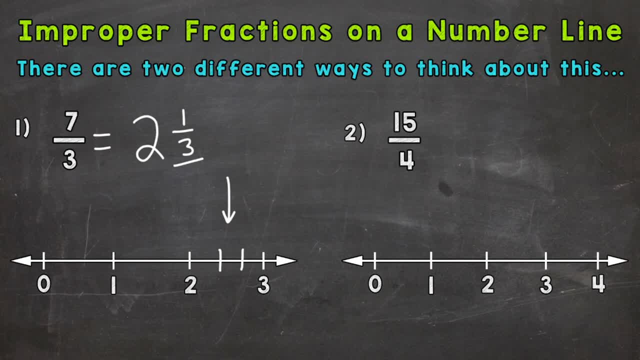 So let's split into thirds here, And this mark here is two and one third, And then we have two and two thirds. Now two and three thirds would be our next mark, This three right here: two and three thirds, Because three thirds is equivalent to one hole. 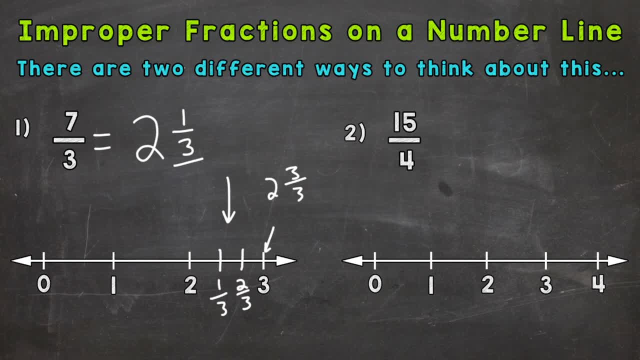 So two plus that one hole would give us three. So if we take the denominator and the numerator, it equals one hole. So our given fraction, or mixed number, is seven thirds, or two and one third, which would be right there. Now the other way to think of it, like the top of your screen says, there are two different ways to think about this. 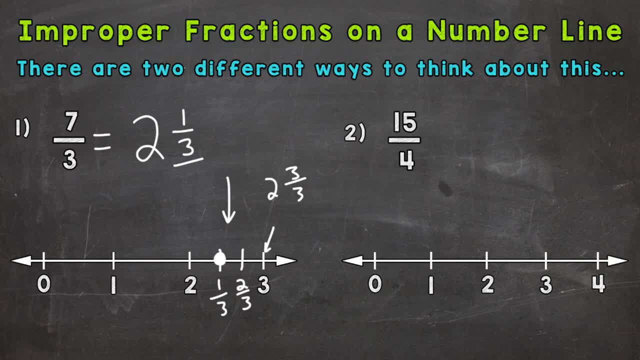 Well, we could go straight from seven thirds. Let's cut the rest of the number line in thirds. between the whole numbers Here would be one third, two thirds, three thirds, four thirds, Five thirds, six thirds and seven thirds. So we end up at the same place, right here. 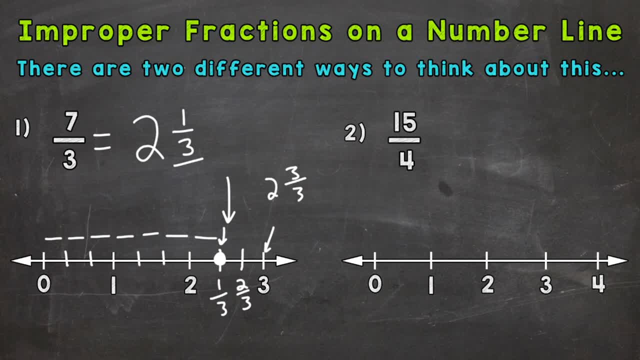 And that makes sense, because seven thirds is equivalent to two and one third. So on to number two, where we have fifteen fourths, And the first thing we want to do is convert to a mixed number. So how many whole groups of four out of fifteen?